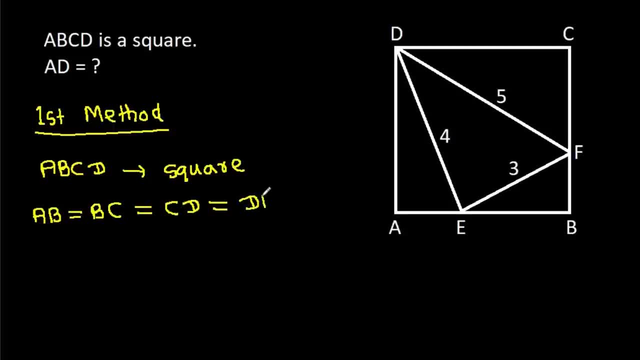 it will be equal to CD. it will be equal to DA. Suppose X, DA is X and AB is X. And now interangle DEF. it is DEF, DE is 4, EF is 3 and DF is 5.. 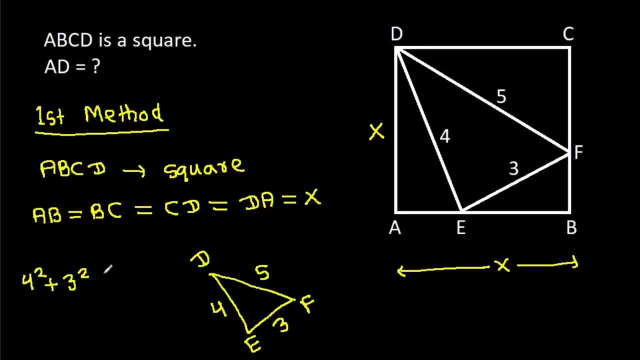 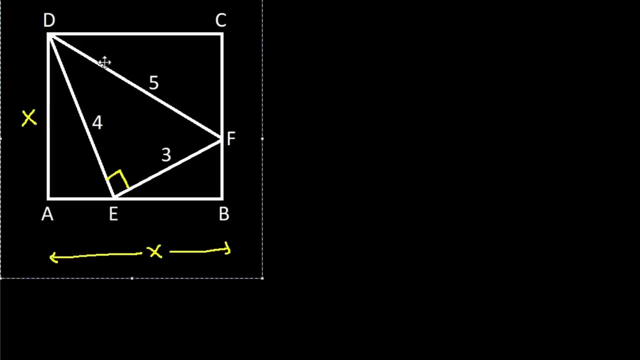 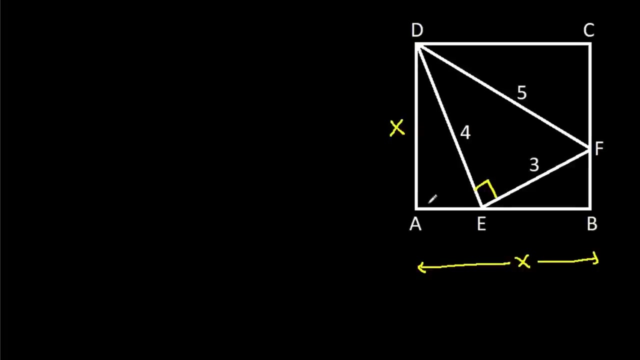 And we know that 4 SQA plus 3 SQA is 5 SQA. that means it will be 90-degree angle. So this angle, it will be 90-degree. And Now suppose this angle is theta. then this angle is 90-degree. so this angle, it will. 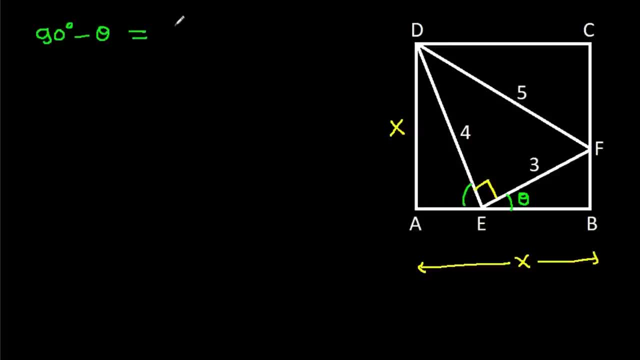 be 90-degree minus theta. suppose it is alpha, then this angle it will be 90-degree. so this angle it will be again theta And this angle is 90-degree degree, so this angle it will be alpha. and now inter angle DAE we have. DE is 4. 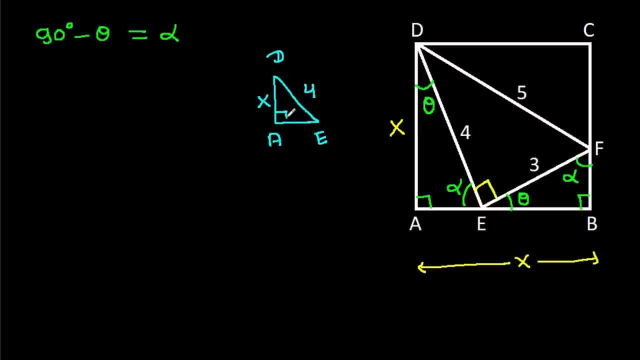 DA is X and this angle is 90 degree. so AE it will be a square root of 4 square minus X square. that will be a square root of 16 minus X square. AE is a square root of 16 minus X square and we have AB is equal to X, so BE it will be equal to. 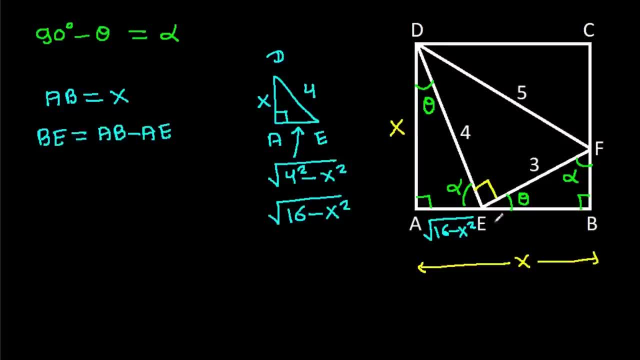 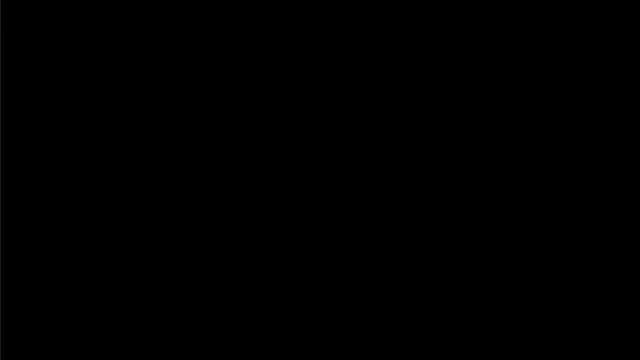 AB minus AE, so BE it will be X minus S square root of 16 minus X square. and now inter angle BAE and Turkey, debf, CE and as a result AB will be equal to AA and Skinn. The calculation is given four, 16 digigt lines in thisfire to x square root؟. 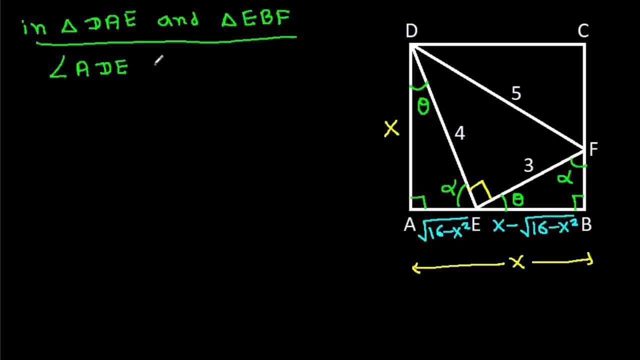 angle ADE is equal to angle BEF, that is theta, and angle DEA it is equal to angle EFB, that is alpha. So triangle DAE it will be similar to triangle EBF. Hence DA by EB it will be equal to DE by EF. 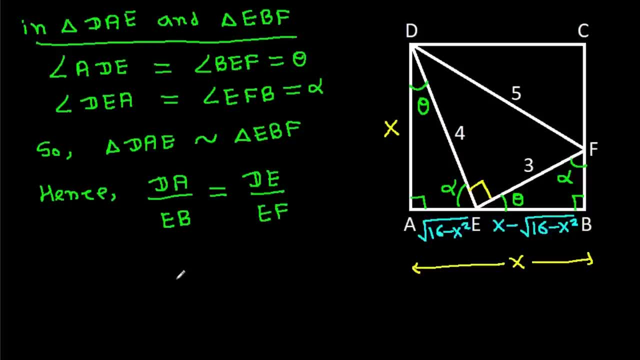 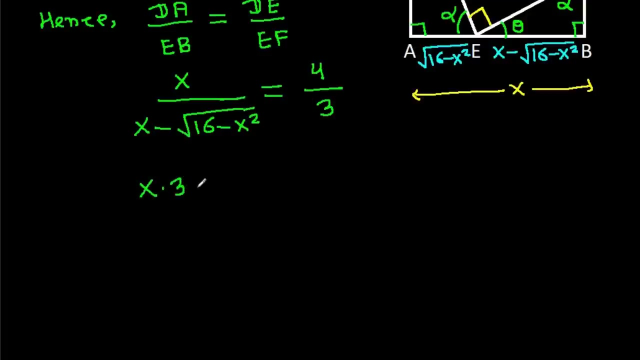 And DA is x by EB is x minus square root of 16 minus x square. It is equal to: DE is 4 by EF is 3.. And if we cross multiply then x times 3 it will be equal to 4 times x minus square root of 16 minus x square. 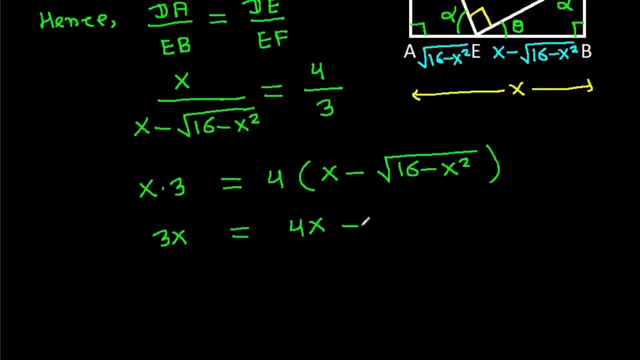 And it is 3x is equal to 4x minus 4 times square root of 16 minus x square And 4 times square root of 16 minus x square. And it is 3x is equal to 4x minus 4 times square root of 16 minus x square, And 4 times. 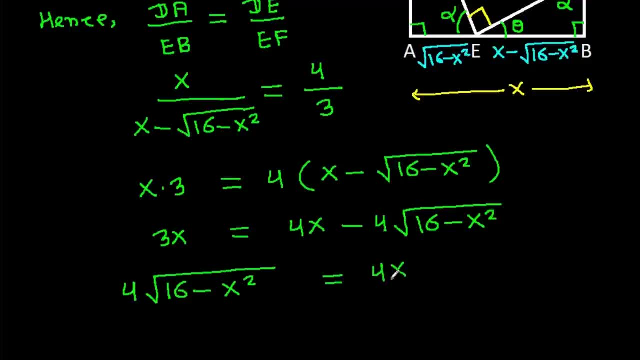 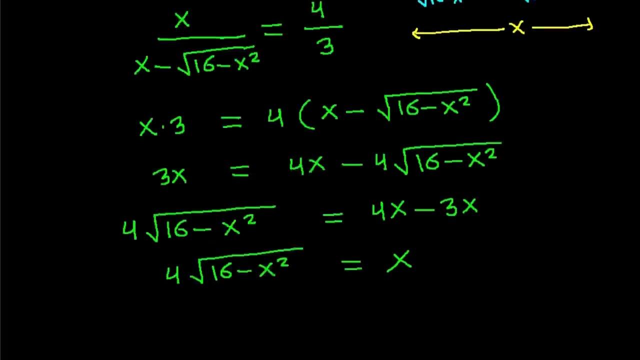 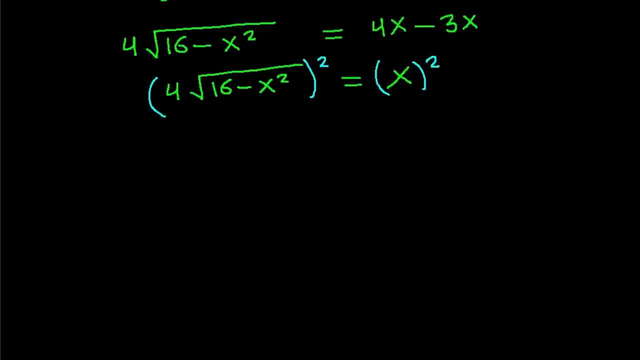 16 minus x square, it will be 4x minus 3x And 4 times a square root of 16 minus x square. it is equal to x And if we square it both sides then it will be 16 times 16 minus x. 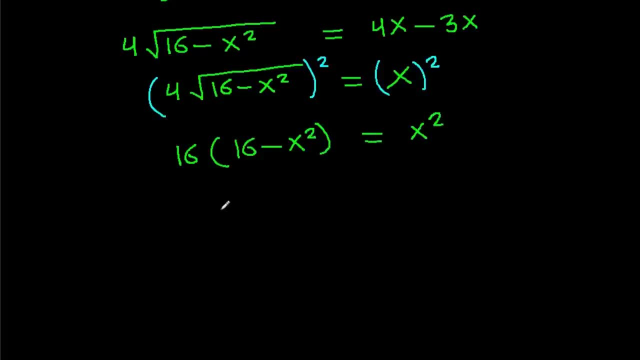 square is equal to x square And it is 16 times 16. minus 16 times x square is x square. So 16 times 16, it will be equal to x square plus 16x square will be 17x square, So x. 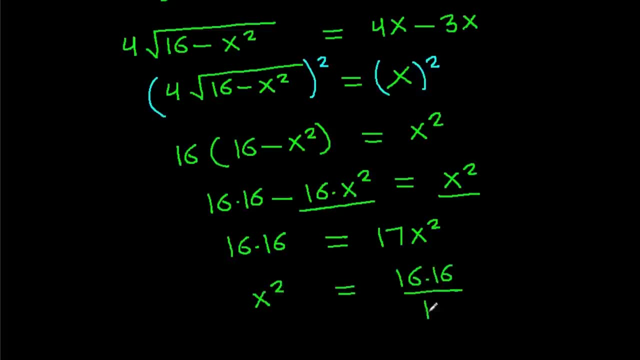 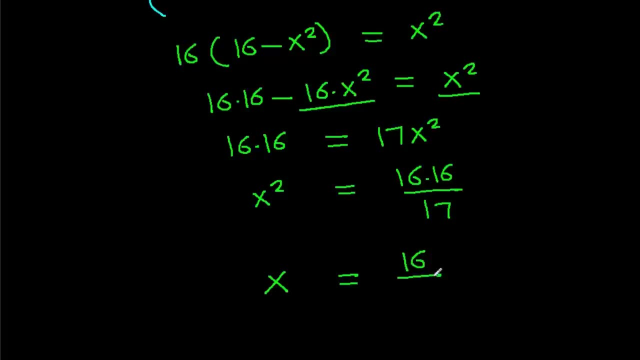 square. it is 16 times 16 by 17.. So x it will be equal to 16 by a square root of 17.. So x it will be equal to 16 by a square root of 17.. 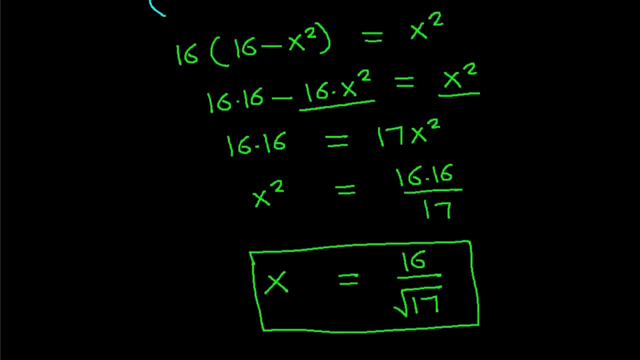 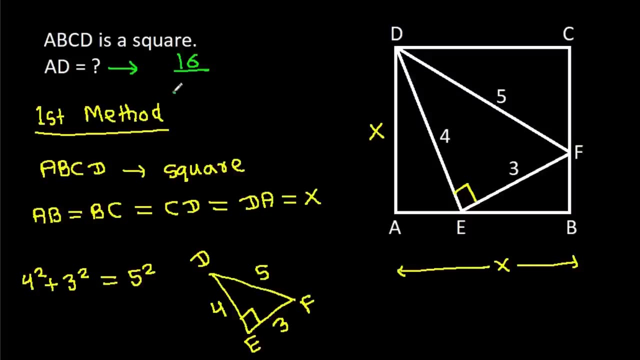 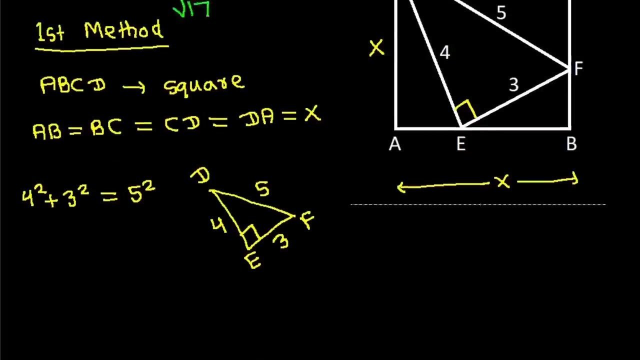 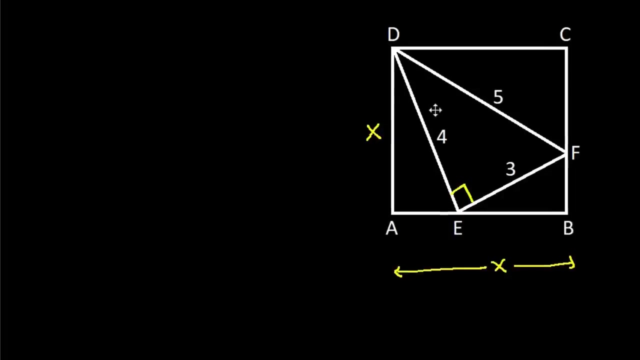 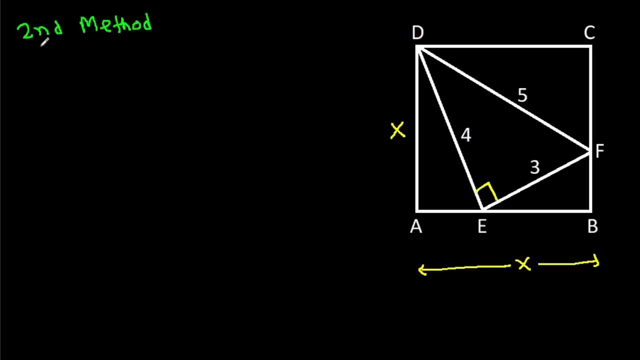 So x, it will be equal to 16 by 17.. So a d, it is 16 by a square root of 17.. And the second method: we know that if this angle is theta, then this angle is 90 degree, then this angle. 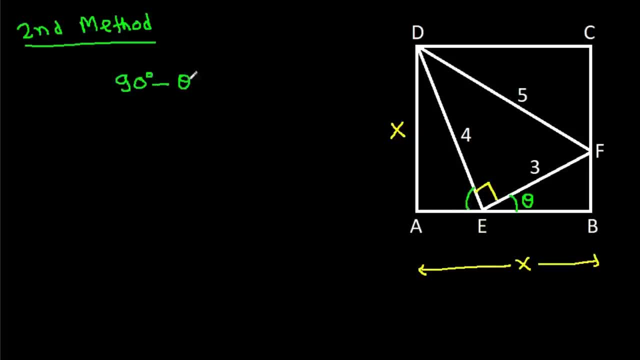 it will be 90 degree minus theta. that is alpha And this angle is 90 degree. So this angle, it will be theta And this angle is 90 degree. So this angle, it will be 90 degree. So this angle. 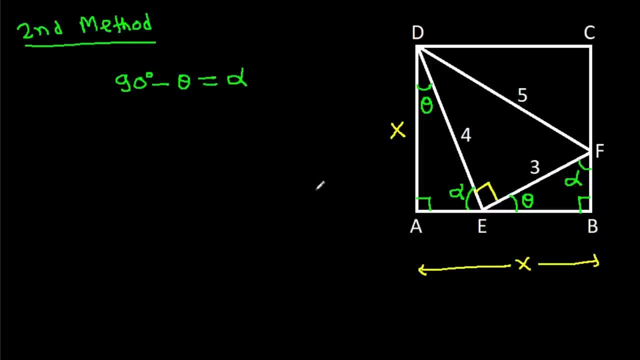 it will be alpha. and now inter angle DAE. we have. DE is 4 and this angle is alpha, so AE it will be 4 cos alpha, AE it is 4 cos alpha and DA it will be 4 sin alpha, so X is 4 sin alpha. 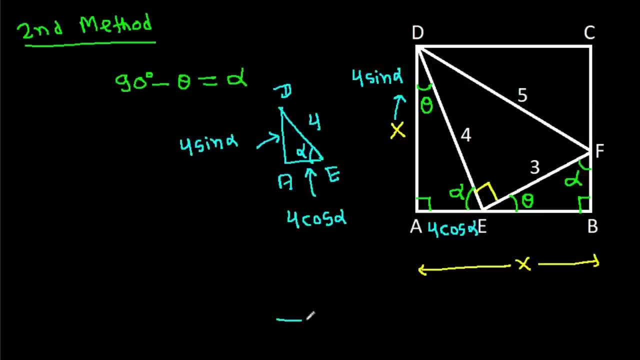 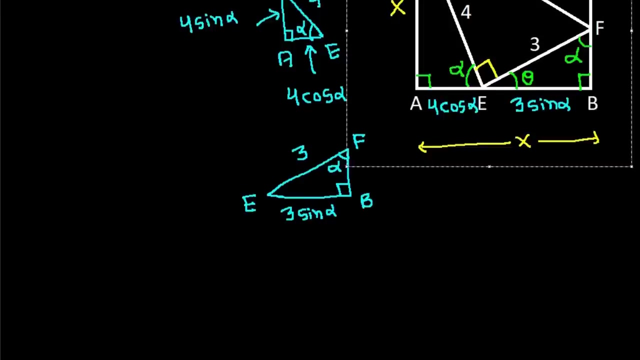 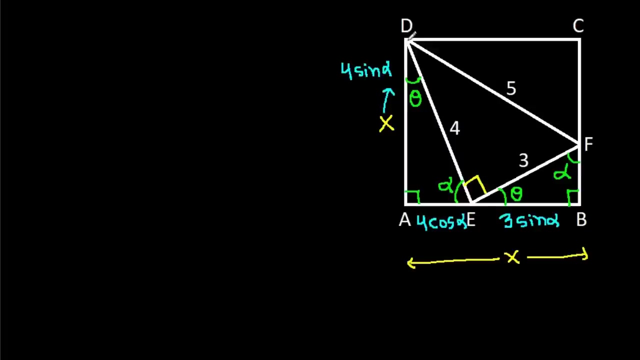 and also inter angle, EBF. this angle is 90 degree and we have EF is 3 and this angle is alpha. so BE it will be 3 sin alpha, BE it will be 3 sin alpha, and, and, and, and. now we know that AD it is equal to AB, that is X, and AD it will be equal to AB, is AE plus BE and AD is 4 sin alpha. now we know that AD- it is equal to AE, is 4 cos alpha. it is equal to AE, is 4 cos alpha plus BE is 3 sin alpha and 4 sin alpha. minus 3 sin alpha it will be sin alpha. that is 4 cos alpha. 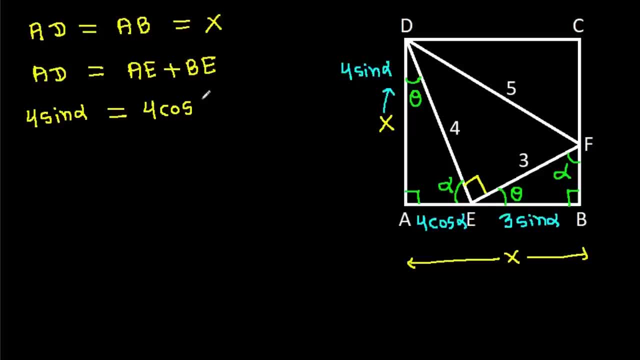 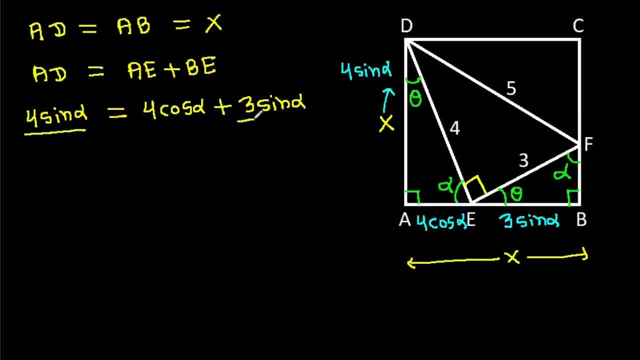 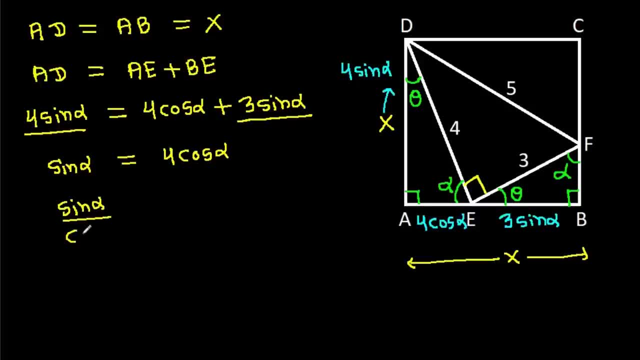 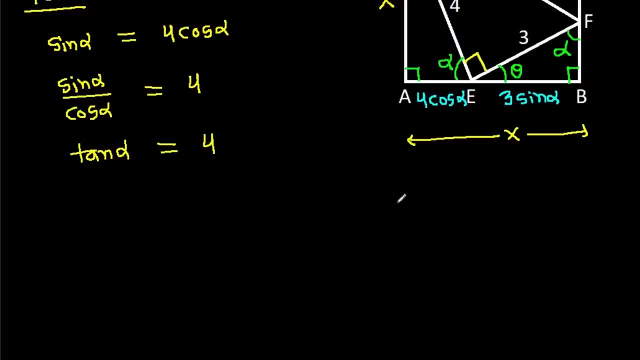 now we know that. now we know that sin alpha by cos alpha it will be 4 and it is tan alpha that is 4. and we know that tan theta, it is P by B and sin theta, it is P by H. That will be equal to P by P is a square.